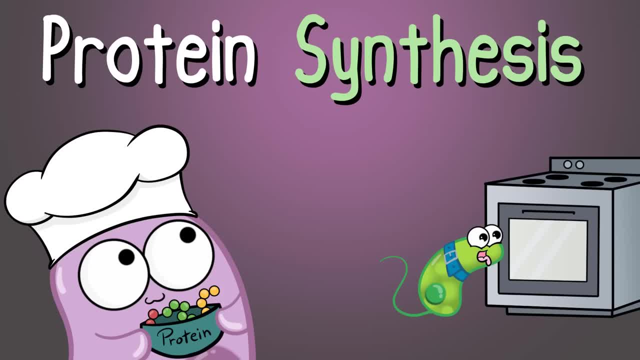 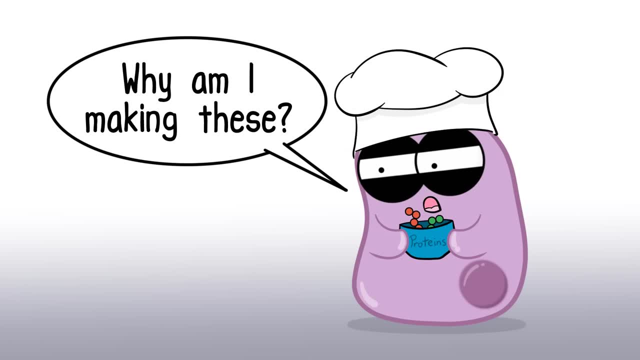 This process is called protein synthesis. Synthesis essentially means to make something. So protein synthesis means to make protein. And you may wonder what's the big deal about proteins. Well, you may not realize this, but proteins are kind of a big deal. 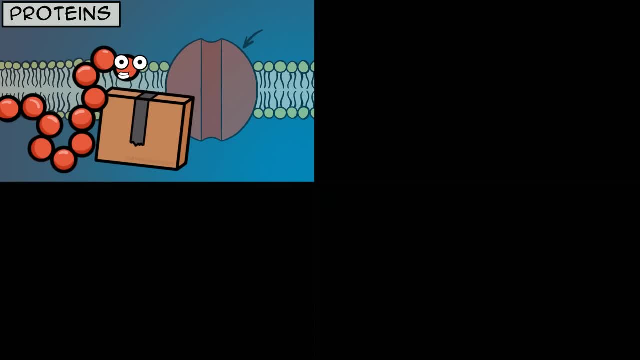 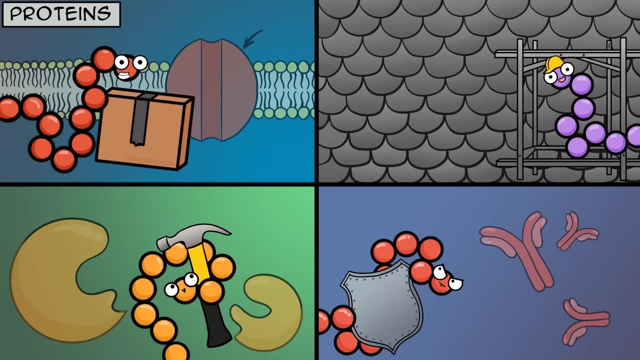 They do all kinds of things. Proteins are involved in transport, in structure, in acting as enzymes that make all kinds of materials, in protecting the body and so much more. You've got to make proteins. It's essential for you to live, And what? 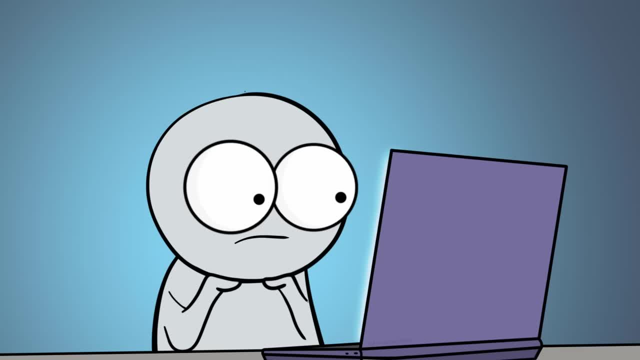 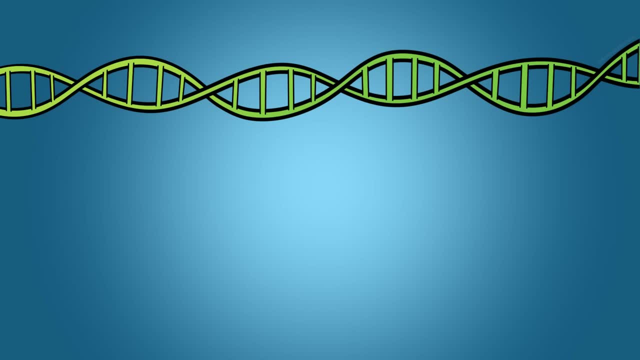 is so cool is that you are making proteins. right now, as you sit and watch this video, It's happening in your cells. They're making proteins. So back to your DNA and its role in all of this. All of your cells have DNA. Well, a. 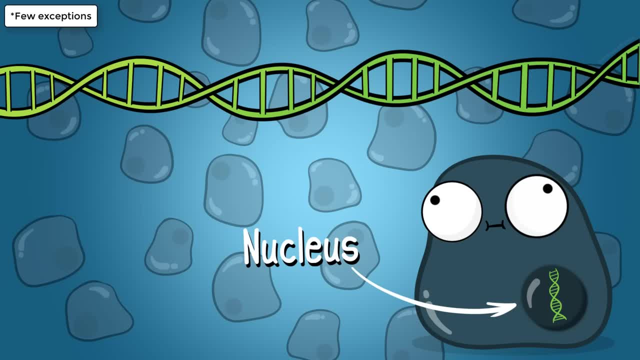 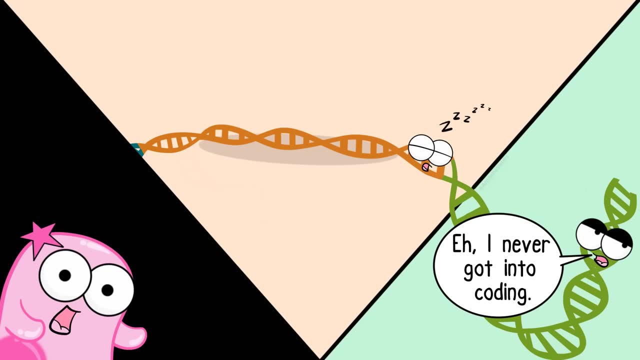 few exceptions, And that DNA is in the nucleus. Some DNA is non-coding DNA, So you're going to make proteins. Some DNA makes up genes that are not activated- More about that in our gene regulation video. But we're going to talk about genes that are coding for active 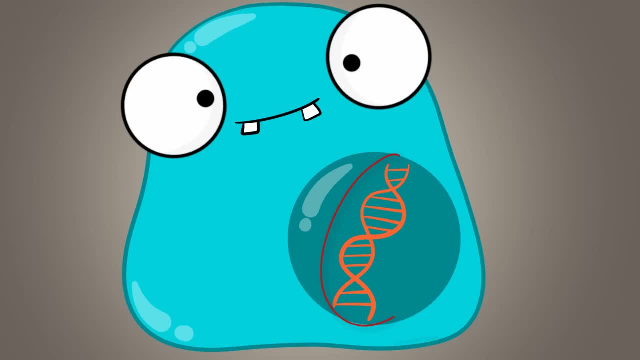 proteins. So how are we going to get the information from these genes out of the nucleus so that the cell can start producing the proteins that it needs to make? Well, let us introduce you to the amazing work of RNA. We have a video comparing and. 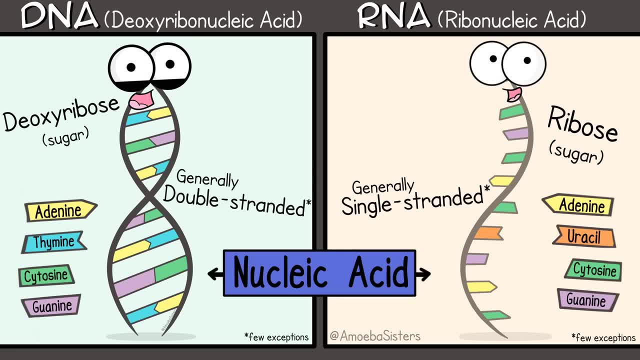 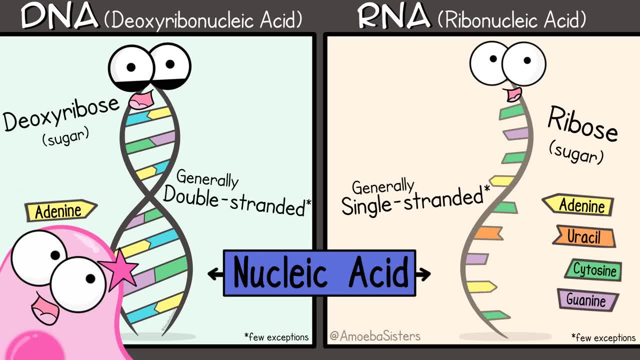 It's a nucleic acid. It's a nucleic acid And it's a nucleic acid like DNA, But it has a few differences. Its role in protein synthesis is also huge. Before we get into the process, please note our typical disclaimer: we tend to simplify. 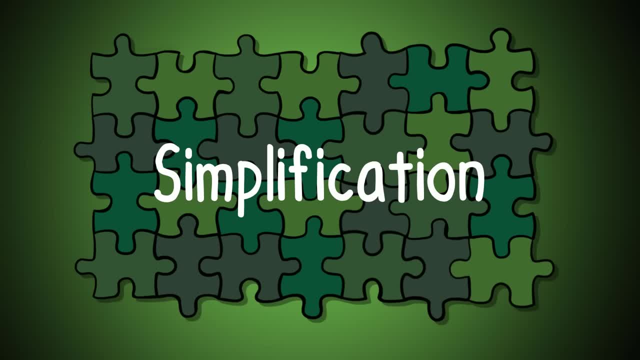 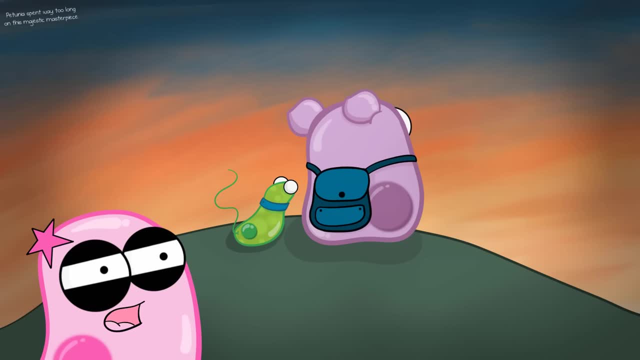 topics, but, as always, if you have the desire to explore this complex, amazing process, later on we hope that you will have the desire to learn all about the extra information that we can't include In protein synthesis. we can look at two major steps. One is transcription and another is 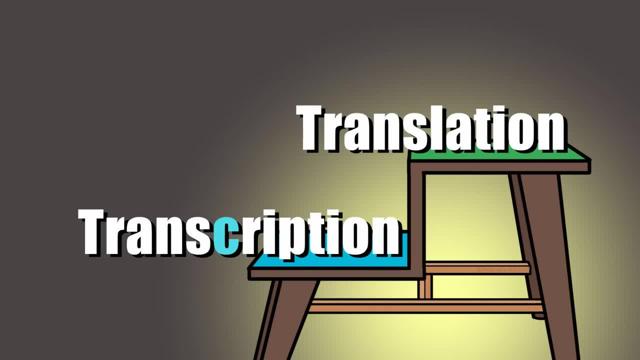 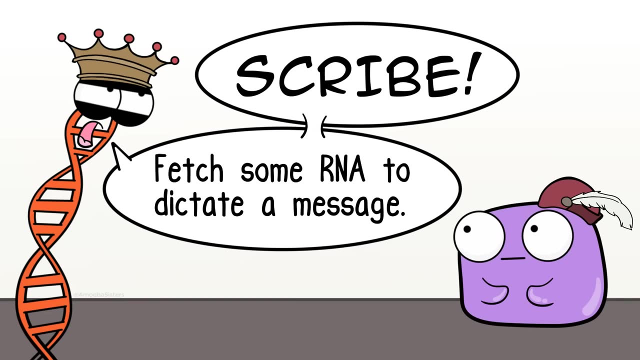 transmission is translation. Transcription has a C in it and translation has an L in it. I remember that C comes before L in the alphabet, which helps me remember that transcription comes first. I like a lot of alphabet mnemonics. Now, transcription is when we're going to transcribe the DNA into. 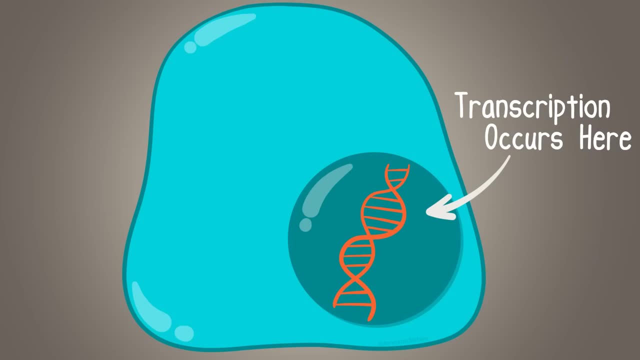 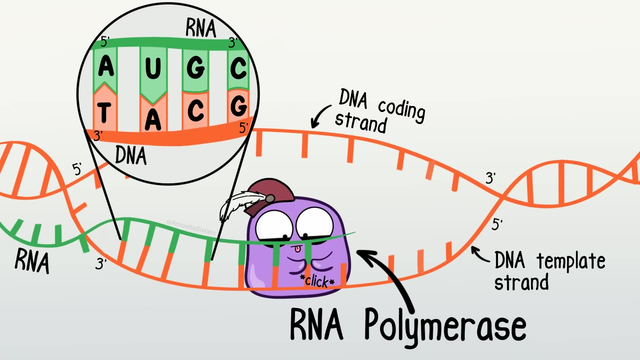 a message. In your cells, the DNA is in the nucleus, so therefore we're doing transcription in the nucleus. In the step of transcription, an enzyme called RNA polymerase will connect complementary RNA bases to the DNA. These RNA bases are bonded together to form a single-stranded. 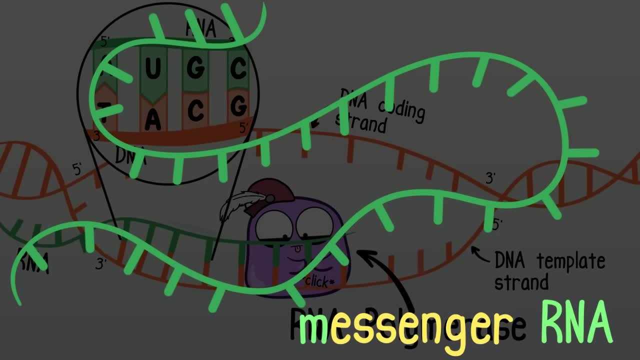 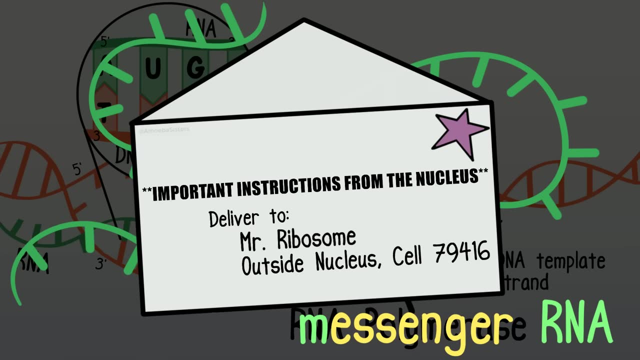 mRNA. The M in mRNA stands for messenger. Messenger RNA consists of a message made of RNA that has been based on the DNA. We do want to mention that this mRNA is not usually ready to go right away. There's usually a signal that the mRNA is not ready to go right away. There's usually a signal. 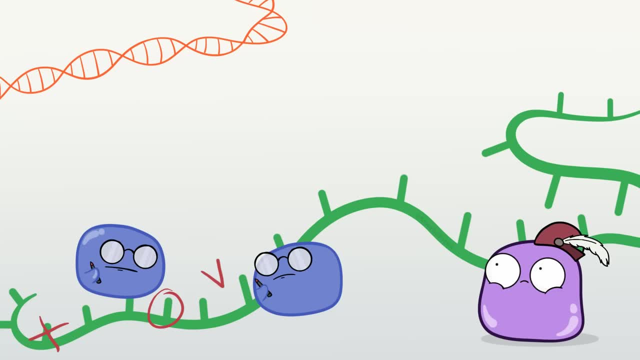 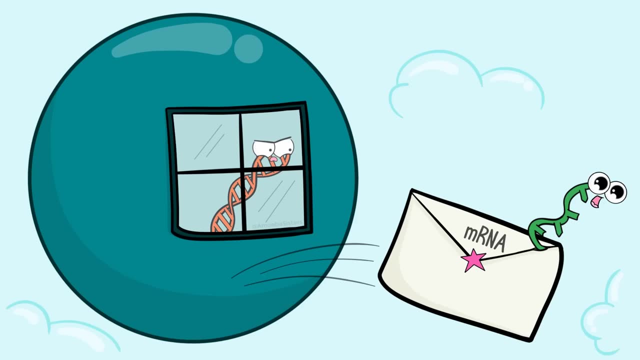 that the mRNA is not ready to go right away and there's a significant amount of mRNA editing that occurs. We highly encourage you to do some reading about that, because it's not only fascinating, it's critical for the process to work correctly. So what's something great about being mRNA? 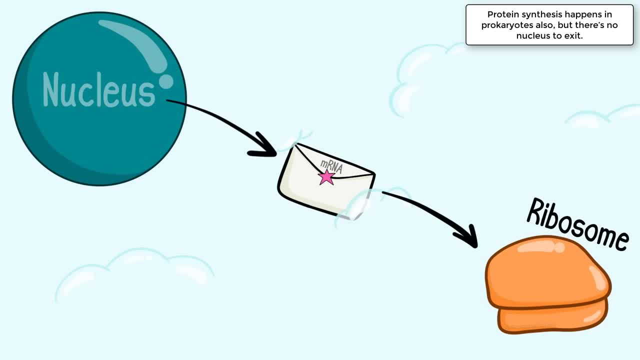 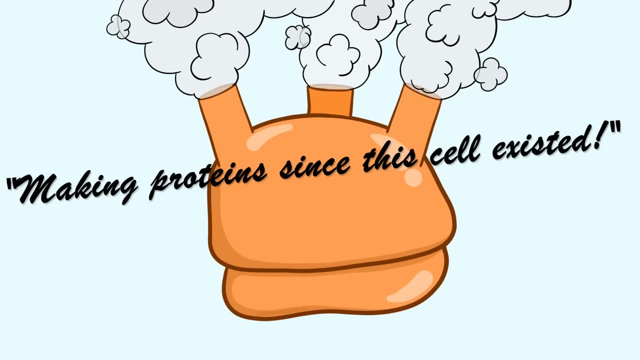 Well, in eukaryotes you get out of the nucleus. The mRNA can go out of the nucleus into the cytoplasm, where it's going to attach to a ribosome. Ribosomes make protein. The ribosome is made of rRNA. That's an easy one to remember, because the R stands for ribosomal RNA. 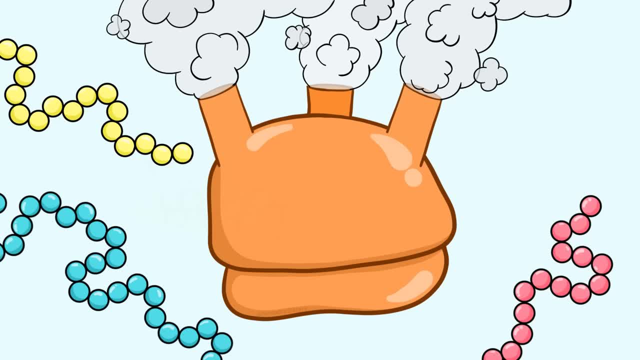 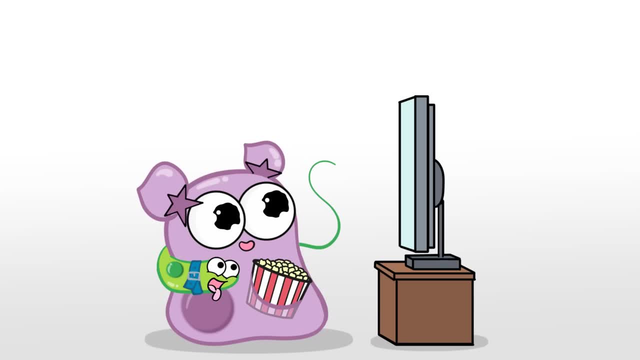 The ribosome is going to build our protein in the next step, called translation. You know you can find a lot of great clips and animations on translation that are just fantastic. We're just going to break down some basics of what's happening. 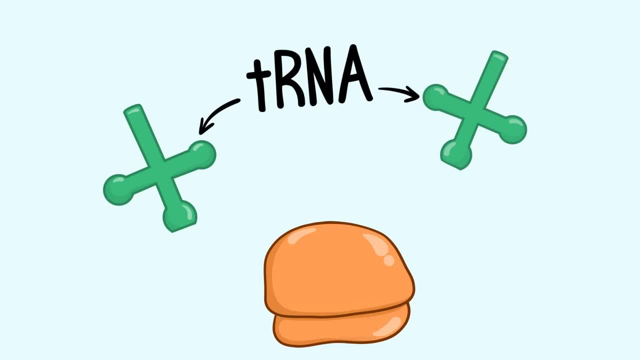 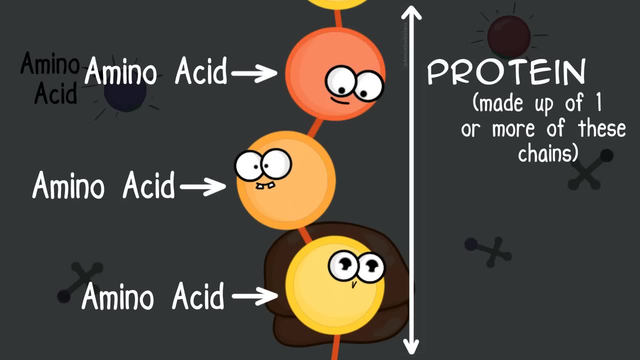 In the cytoplasm. if you look at this, you have all these tRNA molecules available. tRNA stands for transfer RNA. They carry an amino acid on them. An amino acid is the monomer for a protein. It's a building block for a protein. 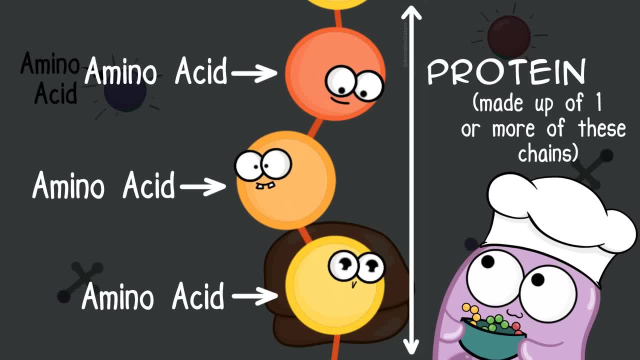 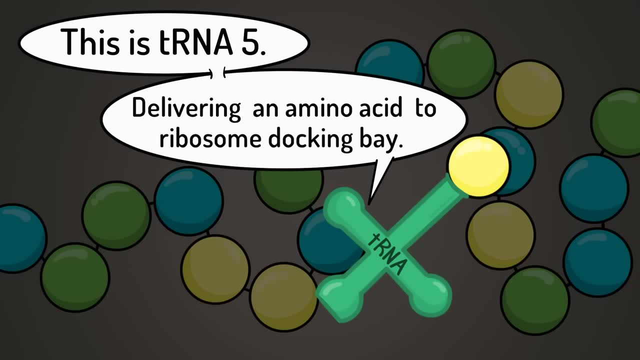 Since we're making proteins, we're going to need those amino acids to build it. If you have a bunch of amino acids together, you can build a protein. So it's the tRNA that is going to bring those amino acids together to make that. 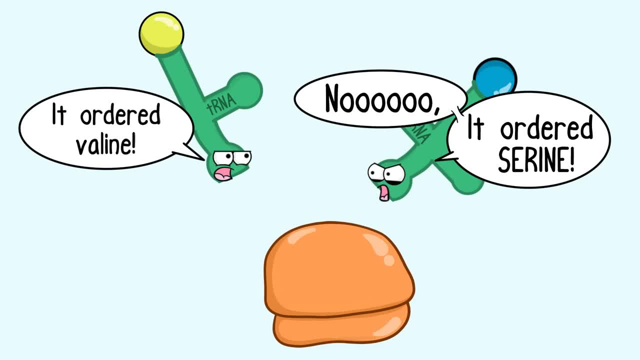 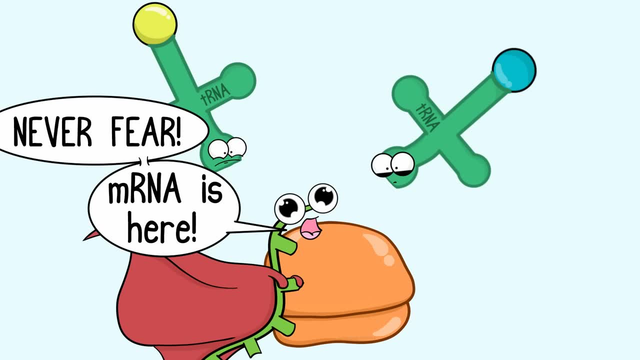 But wait, how does the tRNA know which amino acids to bring? That's why the mRNA. the message is so important, because it's going to direct which tRNAs come in and therefore which amino acids are transferred. All these tRNAs are looking for complementary bases. 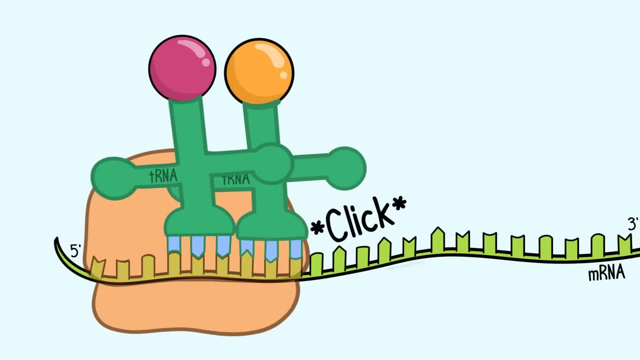 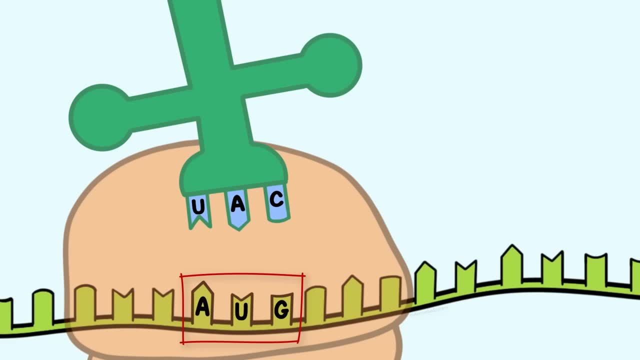 When they find the complementary bases on the mRNA, they transfer their amino acid. When tRNA is bringing in the amino acids, it reads the bases represented by these letters on the mRNA in threes, So it doesn't read one letter at a time, it reads in triplets. 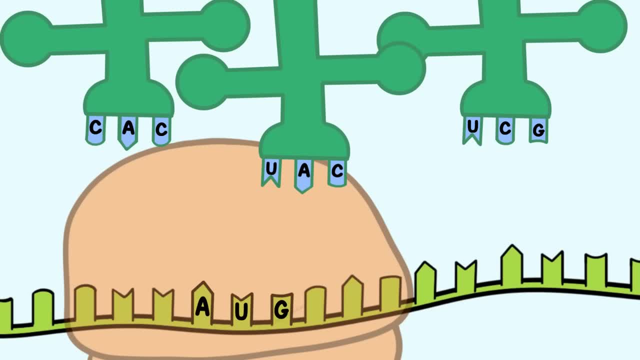 That's called a codon. For example, in this mRNA, the tRNA would read the codon AMYG, The Cart ID of the tRNA iaauftragable. The ASVs are rape Qué Bonajá. One of these tRNAs contains a complementary anticodon, which in this case is UAC. 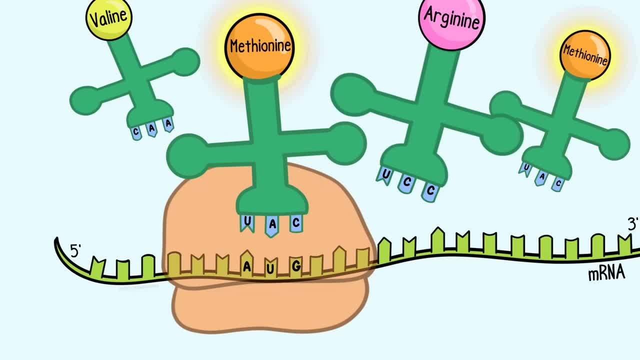 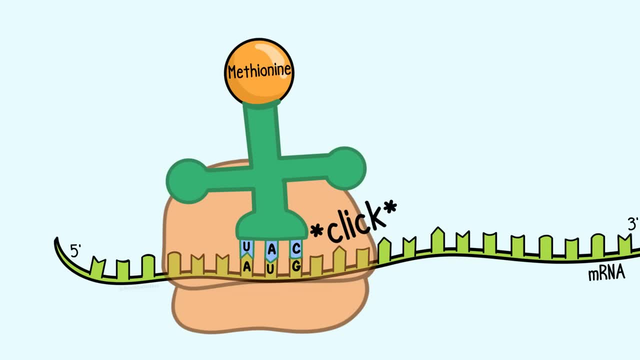 All tRNAs that have the anticodon UAC will be carrying an amino acid called methionine. A tRNA with the UAC anticodon comes in to pair with the complementary AUG codon on the mRNA. It transfers the amino acid. it carries methionine. 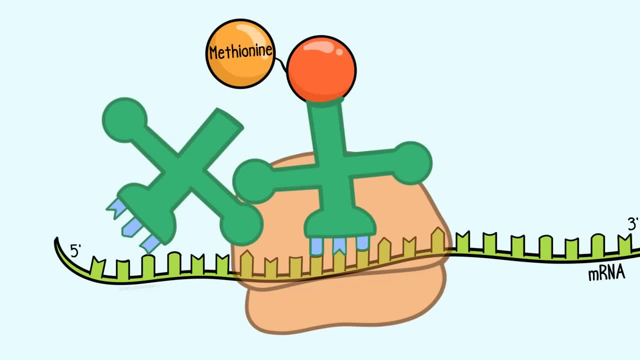 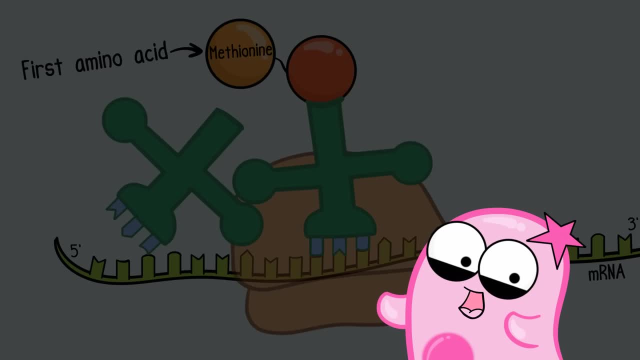 The tRNA will eventually leave, but it will leave behind its amino acid. That's the first amino acid before looking at the next codon, Before we do the next codon to carry this on. if you're wondering, how did you know? 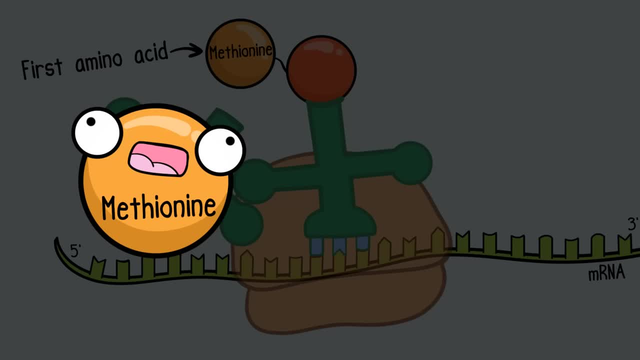 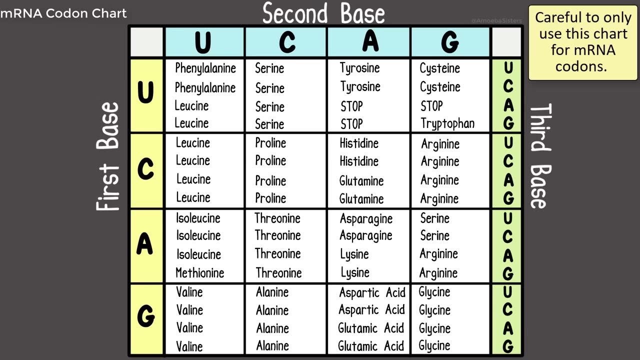 that the tRNA that went with the AUG codon would be carrying an amino acid called methionine. Well, for that you will find a codon chart helpful. You can learn to use a codon chart to determine which amino acid each mRNA codon will code. 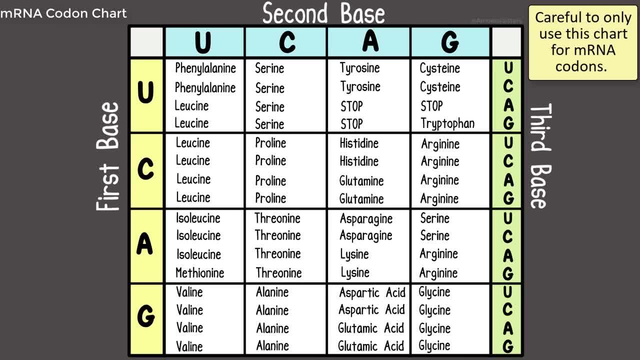 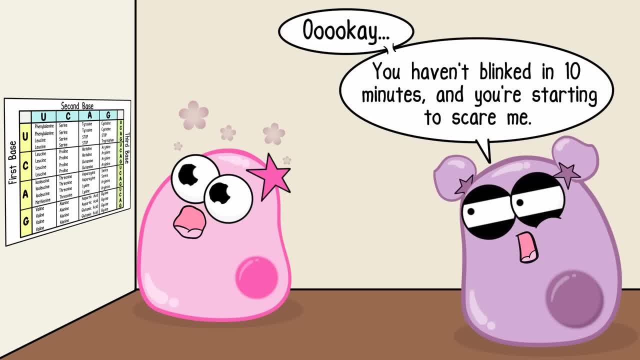 for Isn't it so fascinating that scientists have been able to determine which amino acid corresponds with these codons? I used to have a codon chart poster and just marvel at that. You can see on a codon chart that the AUG codon on the mRNA codes for methionine. 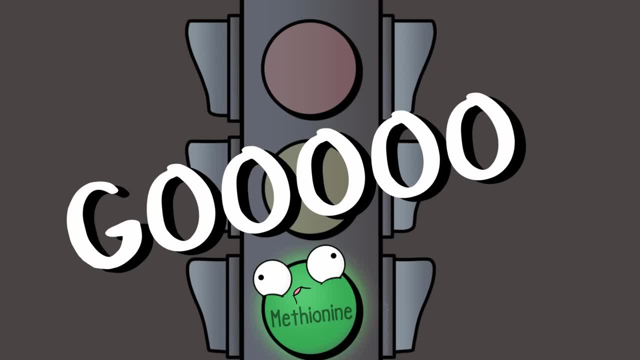 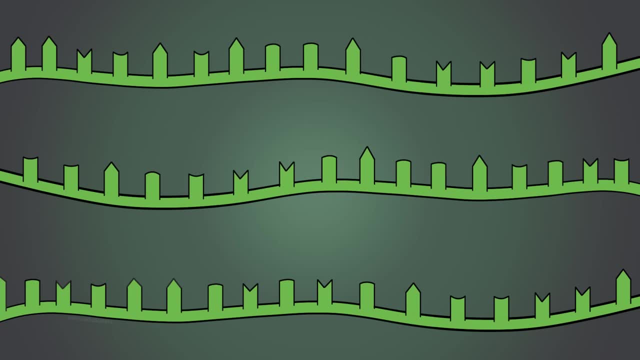 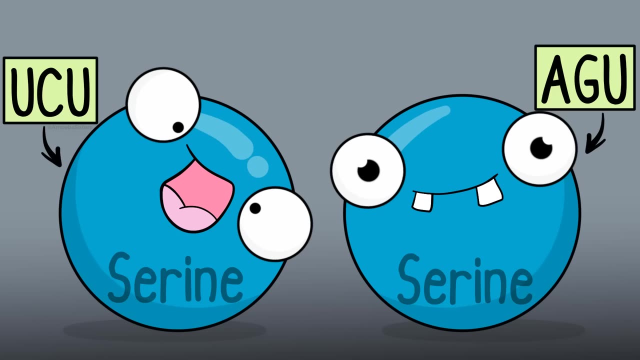 AUG is also considered a start. codon, as methionine, is typically going to be your first amino acid in proteins. There are many types of amino acids in the codon chart, but there are even more possible codon combinations. That means there can be more than one codon that code for the same amino acid.